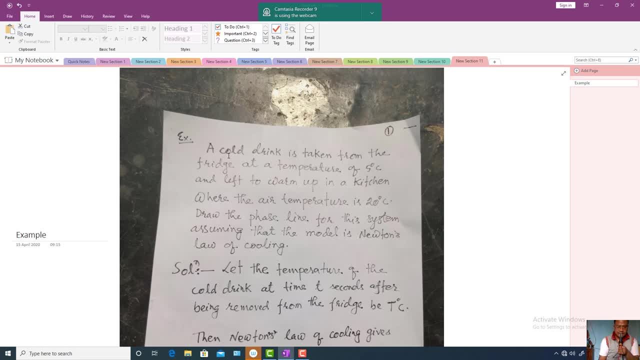 freeze- it is 5 degrees Celsius, and left to warm up in a kitchen where the air temperature is 20 degrees Celsius and then the environment or surrounding area is, you know, temperature is 20 degree, then the temperature of the cold drink will be increasing. means warm up, okay, so that is the thing and how we translate. 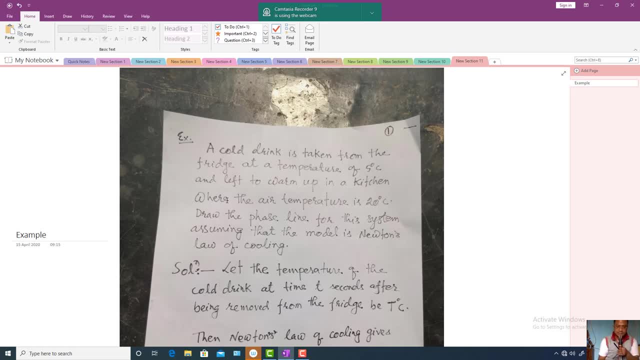 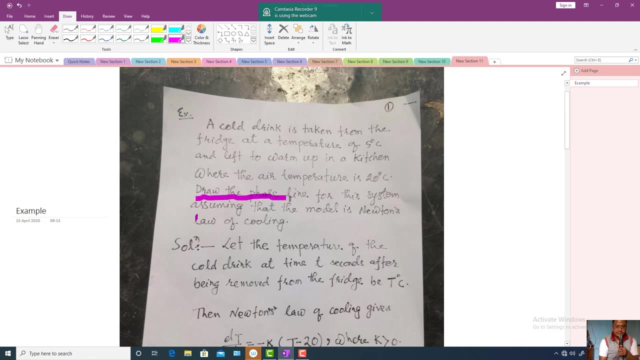 this physical reality world into a mathematical model. so then we see the dynamics. so then draw, you know, draw the face line or face space. okay, for this system, as you mean that the model is newton's law of cooling. okay, so we are assuming here. Newton's law of cooling means the rate of change of a temperature is. 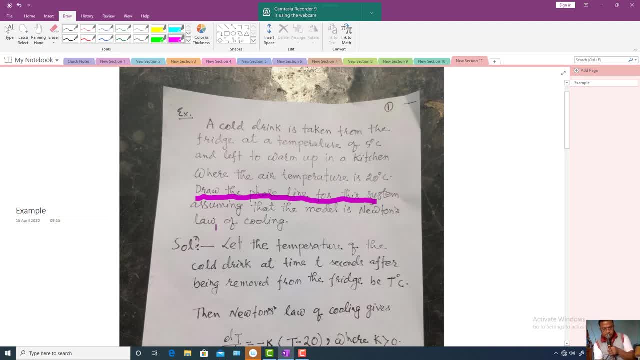 directly proportional to the temperature, the difference of the- you know- temperature of the cold ring and temperature of the surrounding area. okay, so that means if the temperature of the cold ring is cooler than the temperature of the surrounding area, that you know, so the temperature, the temperature of the cold ring will get, you know, warmer, or 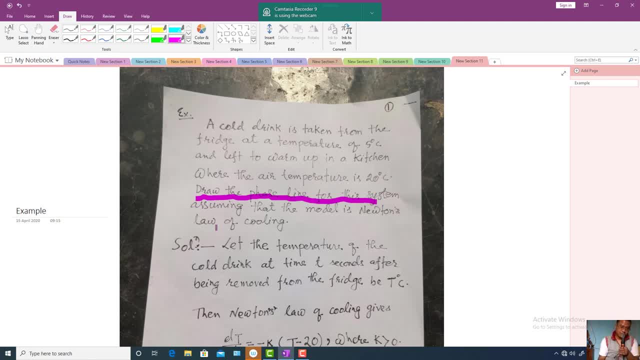 will be increasing if the temperature of the cold ring is more than the temperature of the surrounding area, and then the temperature of the cold ring will be decreasing. so this is the thing we face in the physical world. so so we will translate into you know mathematical model, and according to the Newton's, cooling slow. so, for example, let 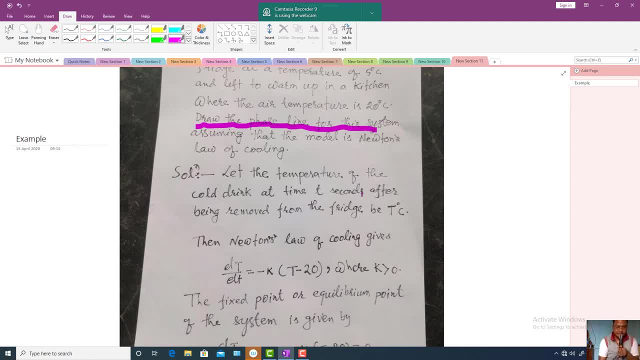 the temperature of the cold ring at a time T second after being removed from the freeze. you know, after, after taken out from the freeze, the temperature of the cold ring will be different, okay, from the original one. so after time T second let the temperature of the cold ring is, you know, capital T degree. 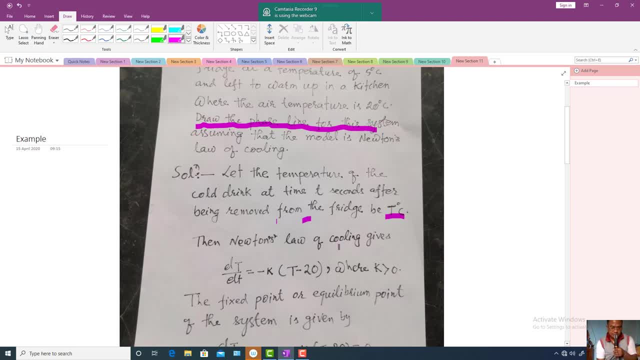 Celsius, then you know, according to the Newton's law of cooling. so the rate of change of the temperature of the, you know this capital, T is temperature, small T is the time there. so rate of change of the temperature of the cold ring is directly proportional to the difference. now, this is, this is temperature of the. 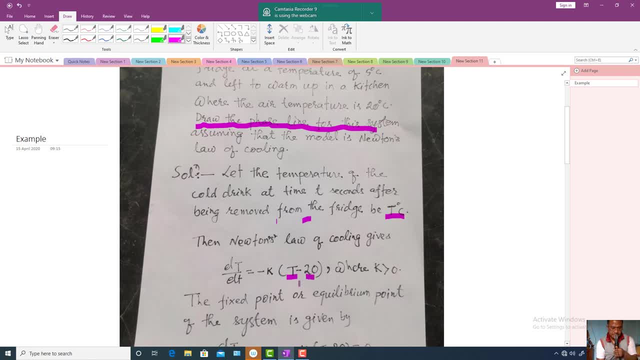 cold ring. this is the temperature of the surrounding area. okay, so so it is multiplied by a constant of you know multiplication K, where case greater than zero. so here we are, you know, putting negative because, because actually so model was for the rate of increase, but yeah, for the rate. 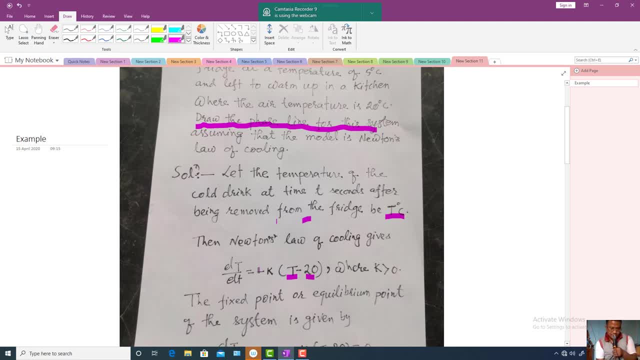 of increase. okay, so the rate of the increase of the temperature of the, you know colding. okay, so later on it will be explained. let us see the fixed point or equilibrium point of the system is given by. you know, the fixed point or equilibrium point of the. 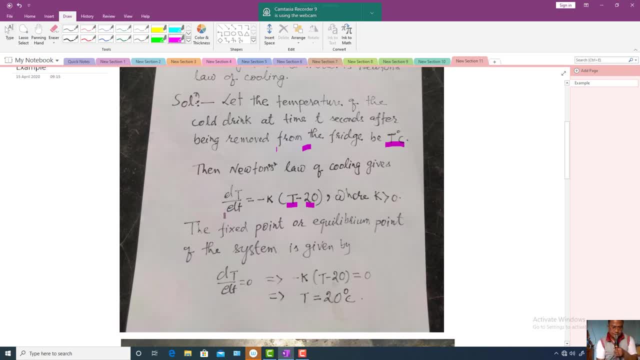 system is given by. you know, when the rate of change of is equal to zero, that we call it fixed point or equilibrium point. so this is the rate of change of. so if it is zero, the solution will give you the fixed point. so temperature T is equal to 20 degrees Celsius, that is the temperature of the surrounding area, or 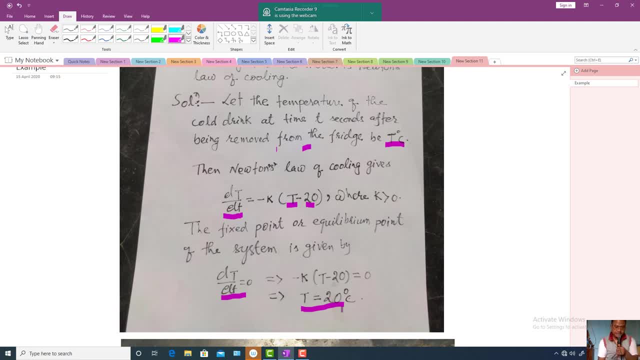 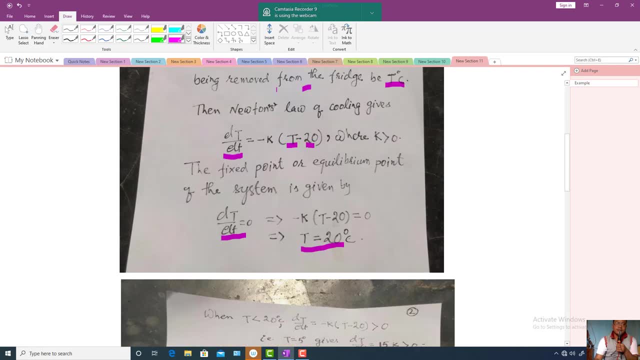 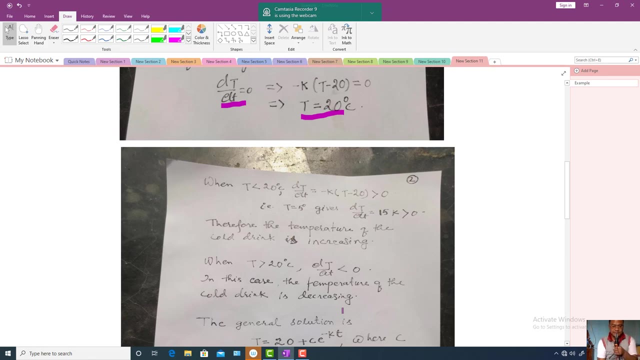 environment or the kitchen is the fixed point. okay, it is the equilibrium point, our fixed point, all right. so, and then let us see when T is less than 20 degree. okay, when T is less than 20 degree, all right. then what so if T is less than 20? 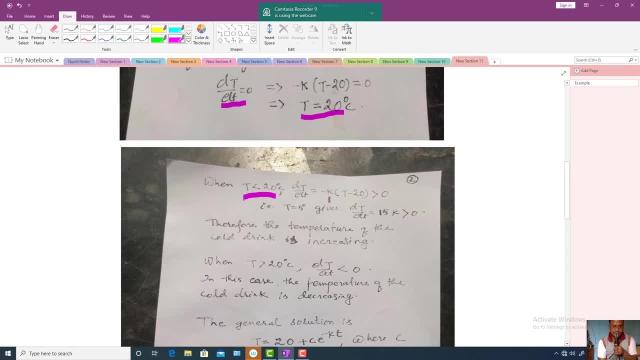 degrees, this is negative. multiplied by another negative, this is positive. so the rate of change is, you know, positive. okay, so one negatives coming from here and another negatives coming from here. then it is, you know, positive. so the derivative is positive, means you know, temperature is increasing, okay. 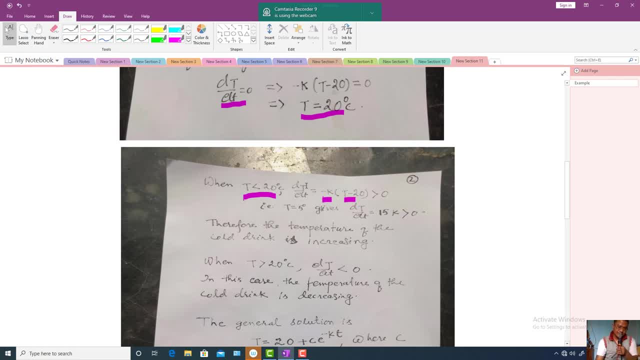 temperature is increasing means you know the solution: function. capital T of this differential equation at this particular temperature will be an increasing temperature function. okay, so temperature increases as time changes, so that is you know when. so if T is equal to 5 degree Celsius, this is less than 20. 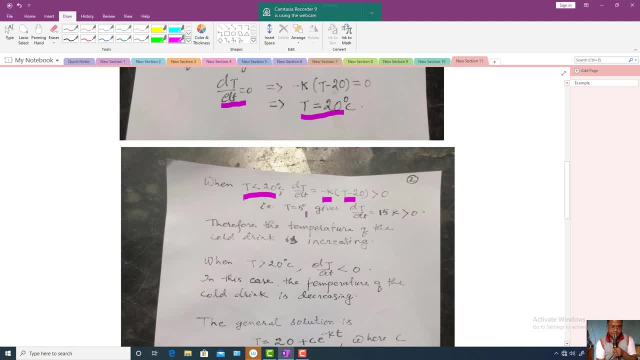 degree. so at the time of, you know, at the time of removing the cold drink from the freeze, the temperature was 5 degrees Celsius. so then, so this mathematical, you know this- analysis of this equation tell us that the temperature of the colding increases. okay, so if T is equal to 5 degree, 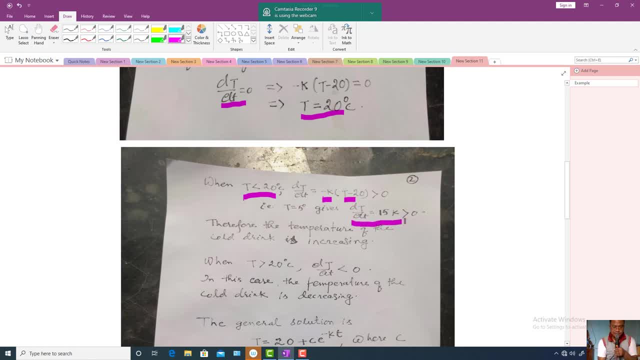 Celsius. the temperature increases is time changes. so therefore the temperature of the colding, okay, is increasing when T is greater than 20 degree Celsius. When T is greater than 20 degree Celsius, Let us see: When T is greater than 20 degree Celsius, Okay, That means you know the cold drink is warmer than the surrounding environment. So in this case it is. you know, DT by DT is less than zero, Okay, So in this case, the temperature of the cold drink is decreasing. 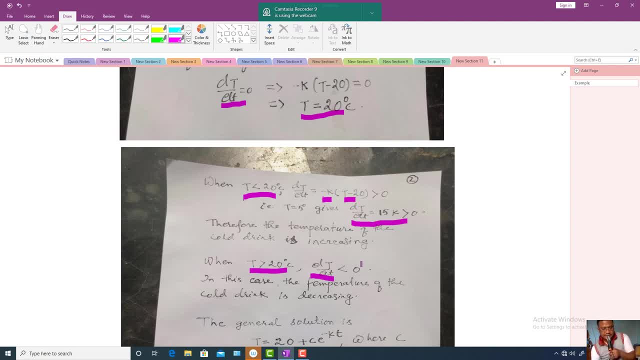 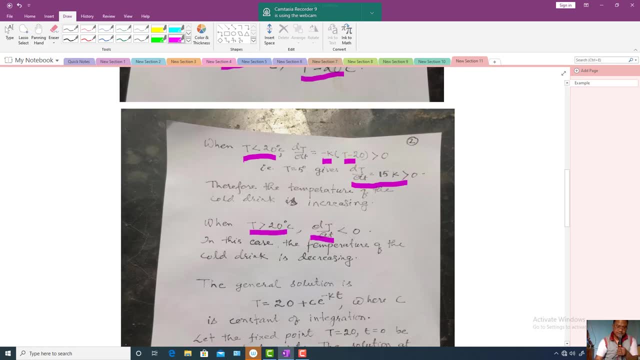 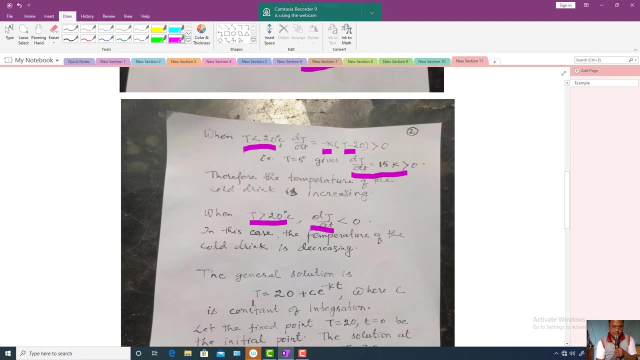 Okay, All right, The temperature is decreasing, So that is the thing. Then let us see the general solution. Okay, Let us see the general solution. The general solution is given by you, can easily solve it. It also satisfies the existence and unit solution of differential equation. So it is easily, you know, solvable. 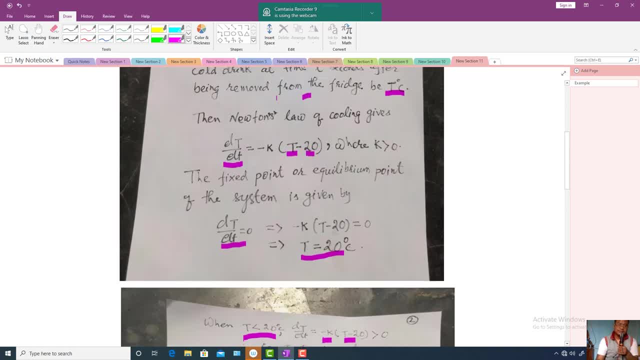 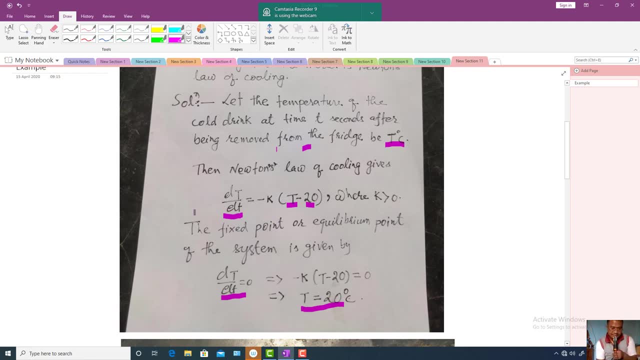 Okay, You can solve it. So let me explain that. the negative part. So it is according to Newton's law of cooling. So, yeah, Cooling means it is decreasing. Okay, Cooling means it is decreasing. So DT by DT, you know, should be negative, Should be negative, Okay, So that is the whole thing. Then DT minus 20 degree The temperature of the surrounding area: Okay, Assume to be, you know, positive. 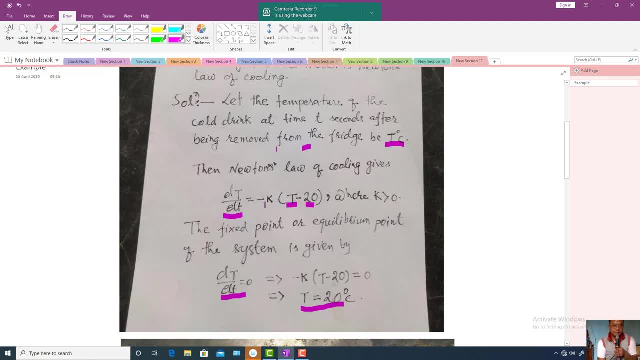 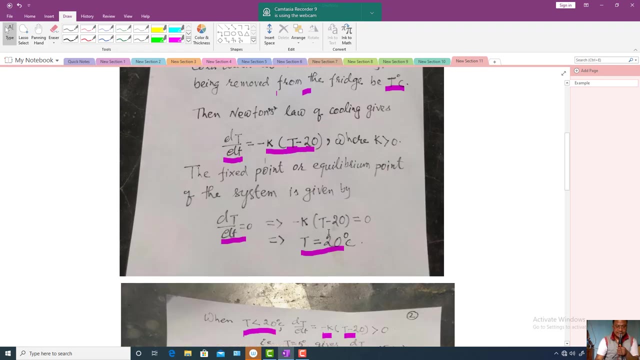 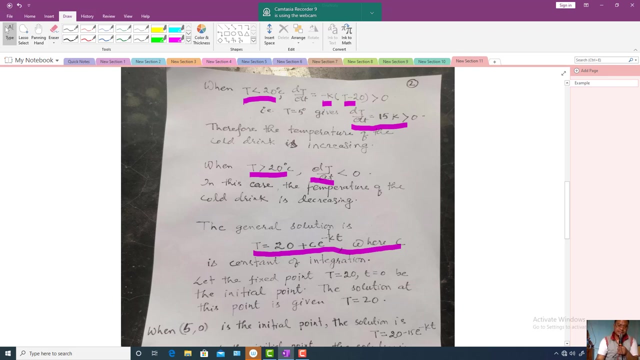 For the time being. So if it is multiplied by negative, So this is, you know, according to the name, it is, cooling means decreasing, So that is why we put here negative. Okay, So that is the. that is the you know explanation, And then you know. So what we have seen is that when the temperature is less than 20 degree, it is increasing. When the temperature is more than 20 degree, 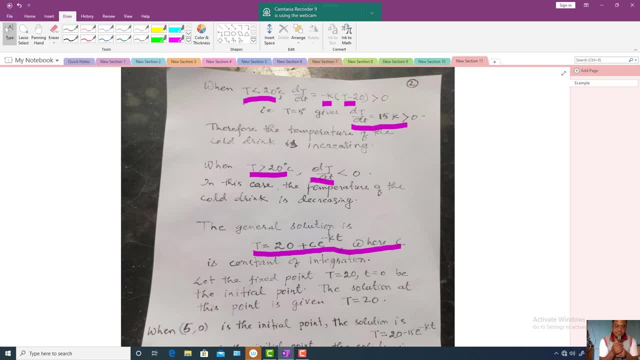 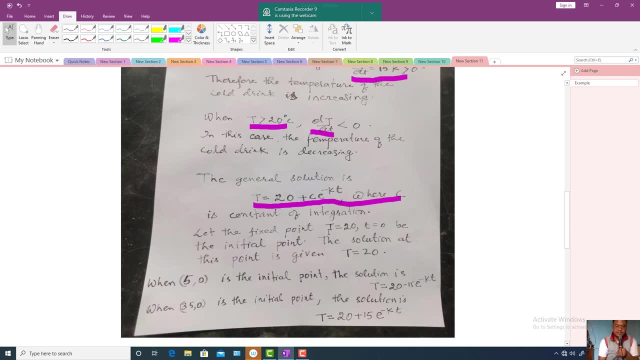 You know It is decreasing. Okay, So, and then the general solution is given by: D is equal to 20 plus, you know, C plus K, E to the power minus KT, where C is a constant, C is a constant of integration. So let the fixed point, you know, let us find out the at the fixed point, what, the what, what, what is the nature of the solution of the given differential equation? Okay, 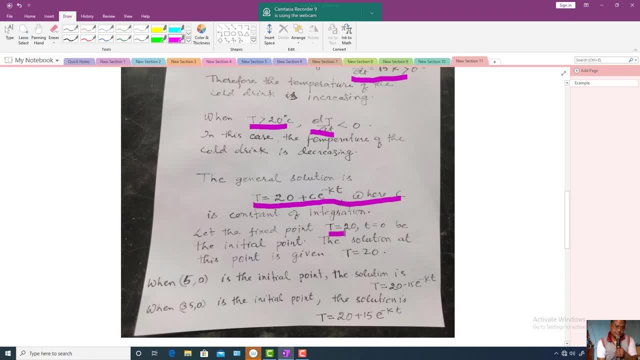 At the fixed point, T is equal to 20.. At a fixed point, T is equal to 20.. You know, let us start the time from there. The moment you take out the freeze, The cooling from the freeze having 20 degree Celsius and surrounding area also is having 20 degree Celsius. So then you know, the common sense say that. what the common sense say, that neither the temperature of the cooling 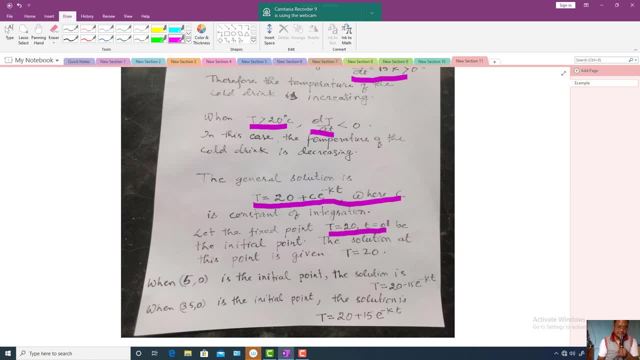 Will increase, Okay, No decrease. It is because he is losing and the temperature is losing. Okay, It is not losing, It is not gaining also. So the thing is that the temperature will be there and it is fixed. That is why it is called, you know, fixed point. It will be fixed When T is equal to zero at the starting point. Let the cooling be taken out from the freeze. 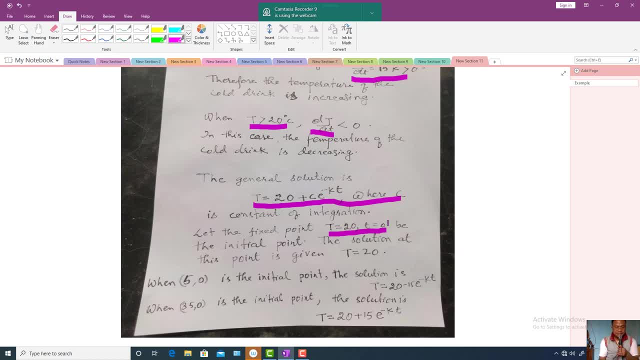 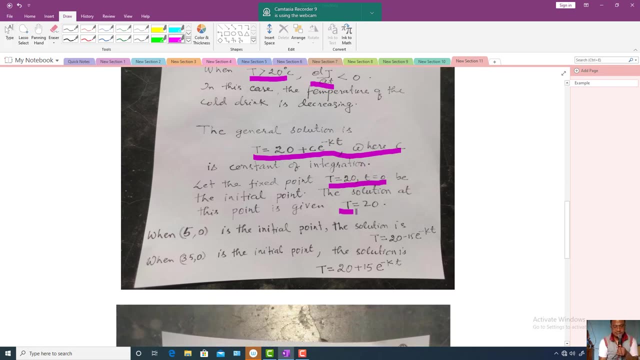 At 20 degree Celsius. Okay, The surrounding area is also having 20 degree And the freeze, The cooling, is also having 20 degree. Okay, So in that situation, the initial value problem. solution of the given differential equation. You can easily say that T is equal to 20 degree. Okay, This is the solution. So differentiate it with respect to T, You will get zero. And then the right hand side, when you put T, is equal to 20. You will get zero, So that this is a solution, Okay. 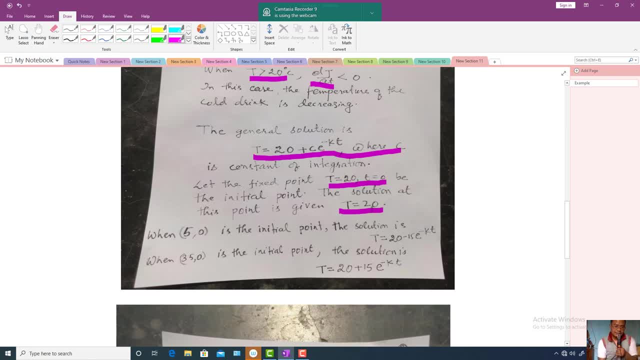 This is a solution. So what does it say? Why we call it is a fixed point? Because temperature is fixed. It is neither increasing nor decreasing. Temperature is fixed. T is equal to 20 degree. Temperature is fixed, Okay, 20 degree Celsius. That is why it is called fixed point. So fixed point, as you know in the earlier, you know in the third semester, Fixed point is very important, If you know. on: 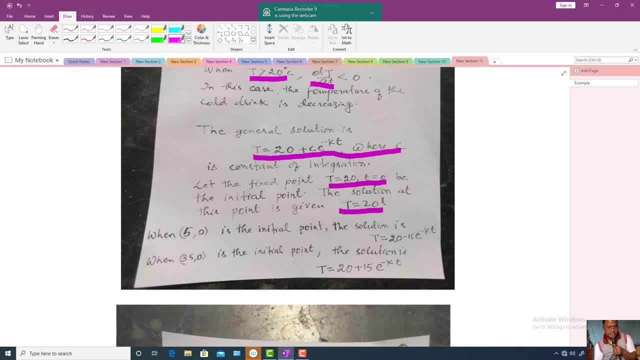 If you know the fixed point Now, on the left and right side of the fixed point, How does the point behave? Okay, How does the points behave On the left and right side of the fixed point In the phase line or phase space? So how does the point behave? Movement of the points or dynamics of the points. So fixed points are very important. So now we have fired out the fixed point And there is only one fixed point. 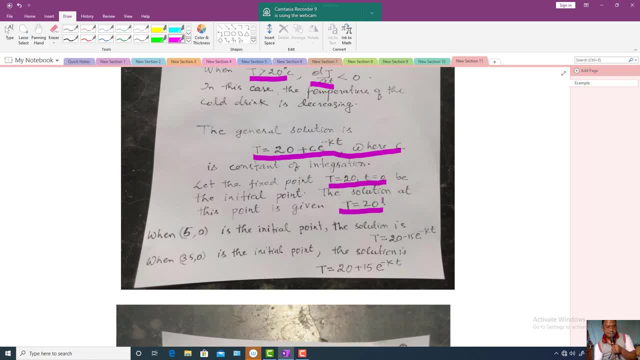 T is equal to 20 degree Celsius. This is the only fixed point. So let us see: 5 degree Celsius is less than 20 degree, So it is on the left of the fixed point: 20 degree Celsius. So when the temperature of the- you know temperature of the cold is 5 degree Celsius, Let us take this is an initial value And time, let us assume the time start from there. So it is the initial value. So solving that. 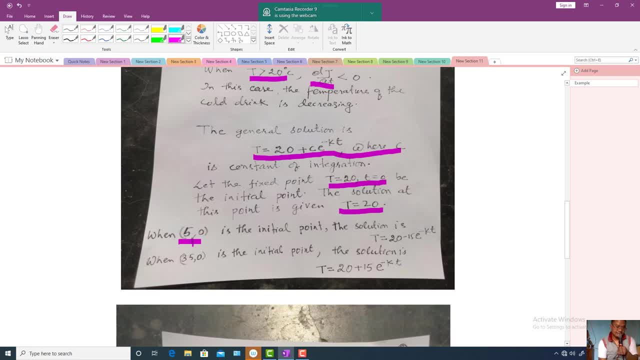 you know we want to solve the given differential equation, or the differential equation whose initial point is 5: 0.. So you can easily solve that one. You will get this. T is equal to 20 minus 15 e, to the power minus k T. You will get this one, Okay. So, and then you know, if you differentiate this T with respect to T, you will get a positive number Right. So that means it is in. 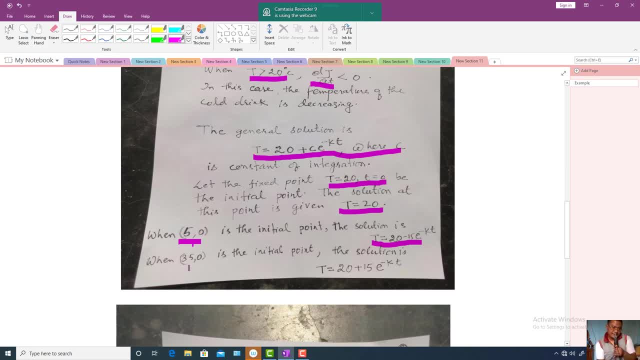 increasing, Temperature will be increasing. So again, let us see when this is the case, when the temperature is less than 20 degree, or that means on the left of the fixed point, Okay. So when, when the temperature is on the right of the fixed point, it is more than the fixed point, that is, 35 degree 0. Okay, Let us just assume that you are taking out the cold drink from the freeze having 35 degree Celsius, Whereas the surrounding area is having. 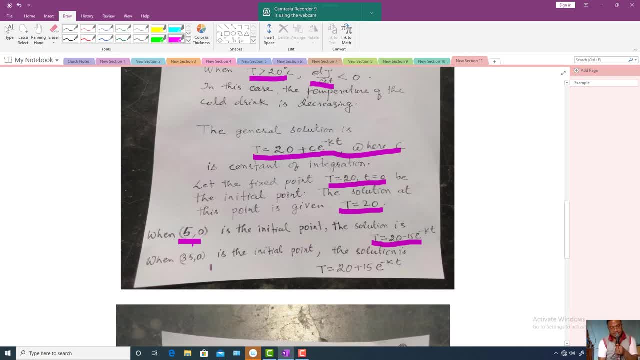 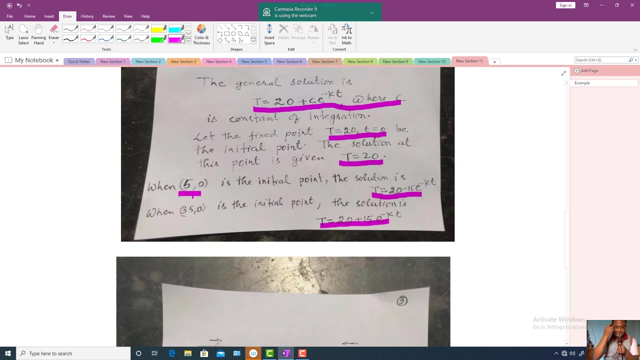 you know, 20 degree Celsius in that situation And let the time start from there. Okay, So in that way, this is the solution. Okay, There will be a unique solution and this is the solution. All right, So this is the solution. Again, if you differentiate it with respect to time and then easily you can check that this is positive, So this is negative, So the temperature is decreasing. The temperature is decreasing, Okay, 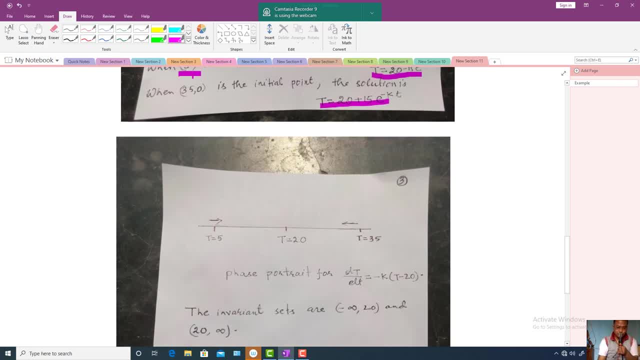 Okay, So let us see, Let us explain it on a, as usual, on a on a phase line or phase space. Suppose this is the phase line, The real axis. the phase line, That means the possible temperature that can be taken out by the. you know the possible temperatures, the, the, the cold drink can take. Okay, So let us assume that the whole real axis is. 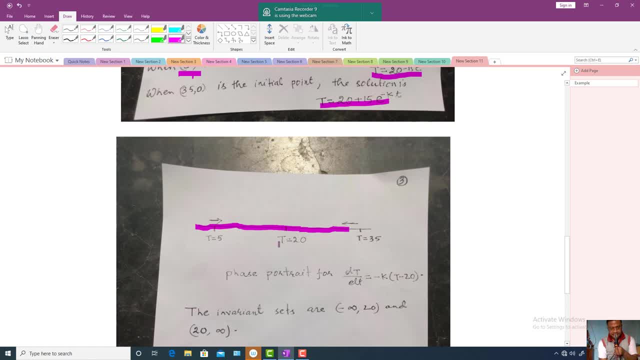 is the phase line When temperature T is equal to 20 degree Celsius. it is here. This is one, this one, Okay, This one. So this is the the fixed point, This is the fixed point. You know, this is the fixed point. Okay, On the left, on the left of this one, temperature is increasing. I am giving one error here. That means all the pose, all the phase points on the left of this 20 degree Celsius. 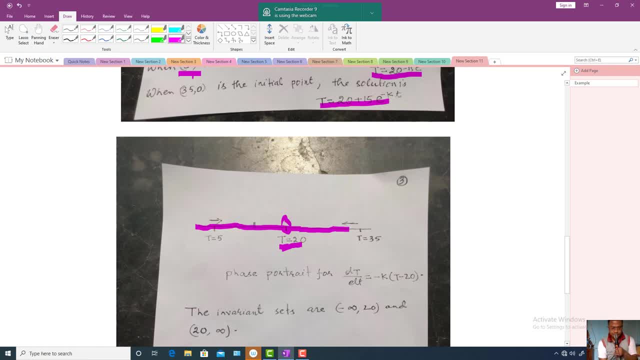 It will be moving. The dynamic behavior is that it will be moving toward the. the fixed point T is equal to 20 degree Celsius. On the right side it is decreasing means all the, all the phase point, or the possible temperature of the cold drink Which is more than 20 degree Celsius. It will be moving this side. Decreasing temperature is decreasing, So it will be moving this way. So, looking at the, you know phase line. 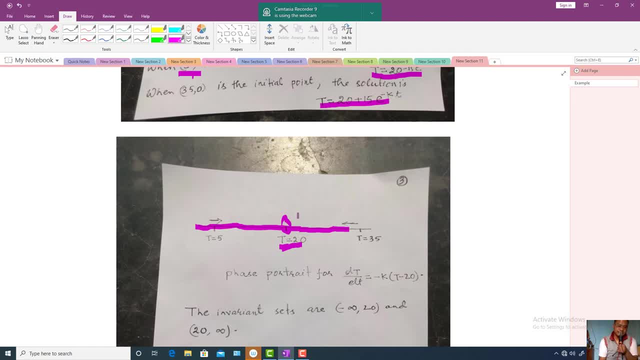 know, if you know the fixed point and the nature of the fixed point. if you know the nature of the fixed point, then how does the phase point behave on the left and the right side of the fixed point? so on the right side the phase points are moving toward the fixed point. okay, that means they are decreasing on the left. 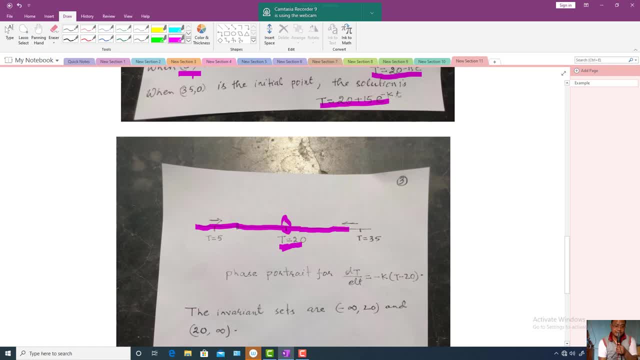 side, the phase points are moving toward the fixed point. that means the they are that it is increasing. okay, so that is the thing. and if you start from a 20 degrees Celsius, it is not moving anywhere. it is fixed point. that is why we call it fixed point. it is neither going this way nor this way. okay, it will. 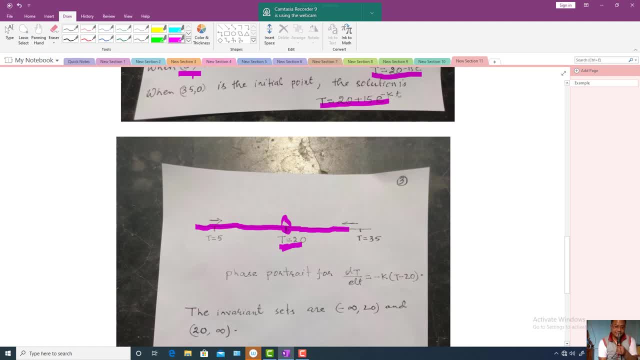 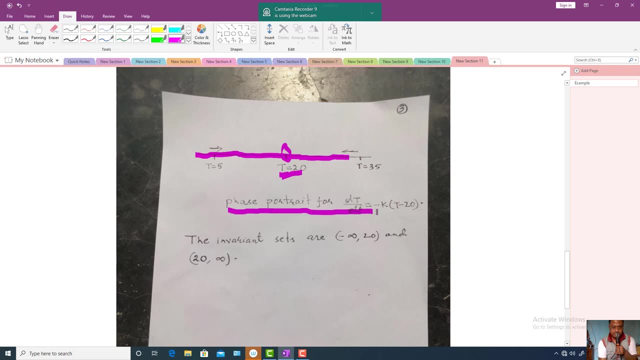 remain here indefinitely, okay, it will be here at all time, right? that is why this point we call a fixed point. so so this is a phase. we call it a phase portrait. you know, in the phase portrait what we do: we find out the fixed point and then 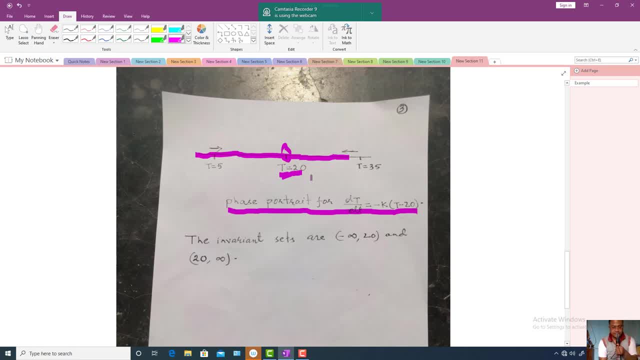 in this case, luckily, we have only one fixed point and then around a fixed point, how does the face point behave? that is the thing. and then we understand: hmm, so then the you know one. suppose you take one temperature here, one temperature here, suppose with 10 degree Celsius. okay, the cold ring, the. 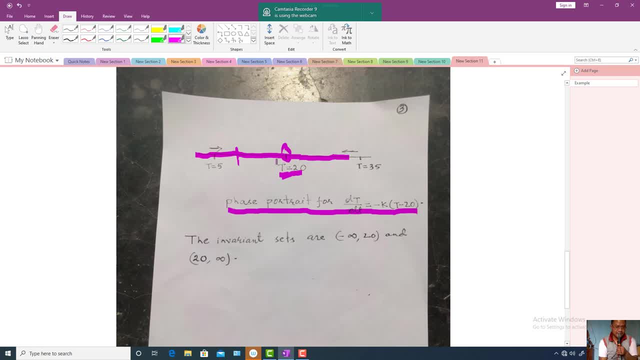 cold ring can take the maximum temperature 20 degrees, it will not across 20 degree. it will never, ever happen that the cold drink temperature will be 25 degree celsius. like that. it will never happen. okay, all right. so again, if the, if the temperature, the 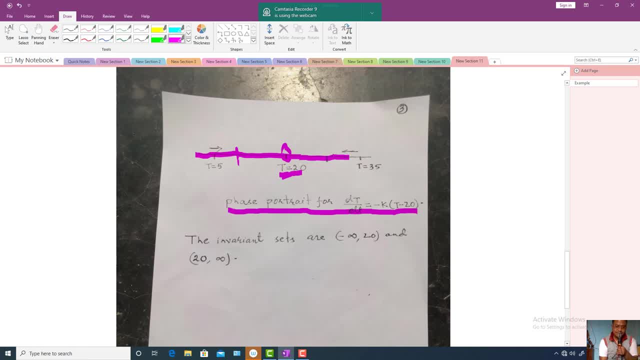 cold drink is say, for example, 35 or 25 degree celsius, it will come down to the 20 degree celsius, but it will not come down below 20 degree celsius. that means, whatever point here on this line, real axis, the positive, you know this one, this axis, okay, whatever point here, it will never cross. 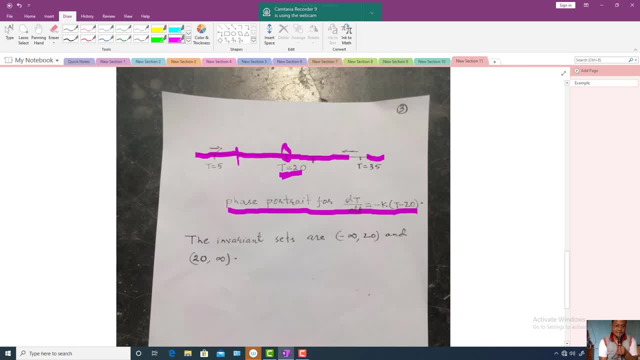 this side. the movement of this point will never cross this side. the dynamical behavior of the point here will not cross this 20 degree, will not cross this line. okay, so that means they, they, the dynamics, you know the movement and of the points always confined in this point. 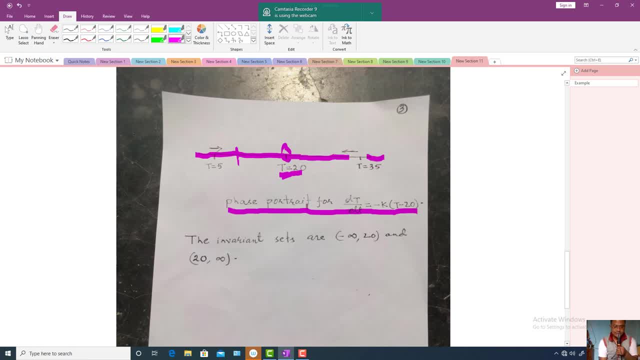 okay, in this, in this part of the real axis that means 20 degree and this one 20, 20 degree to infinity. okay, the movement will be restricted here, only all right. so again, from this side, it will not cross this 20 degree, so the movement will be, you know, restricted this side, this we. 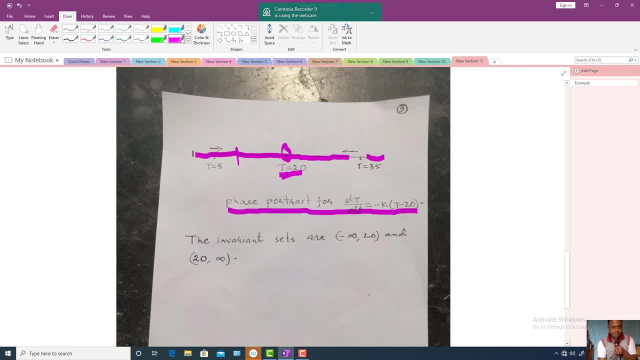 call it. you know mathematics. what we call it? invariant set, all the set of point in this line. you know, on the left side of this 20 degree celsius, their invariant means its image. you know the movement will be within this side only. okay, if you start a point from here, the movement will be. no, the behavior of the points movement is. 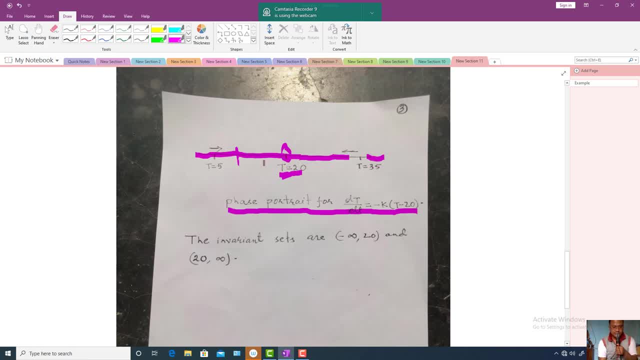 that it will confine in this part of the phase line only. so, like that, from here also, it will be confined on this part of the phase line. okay, that is why it is called, you know, invariant set, invariant set. so invariant sets are always, you know, open set. you know this is open set. 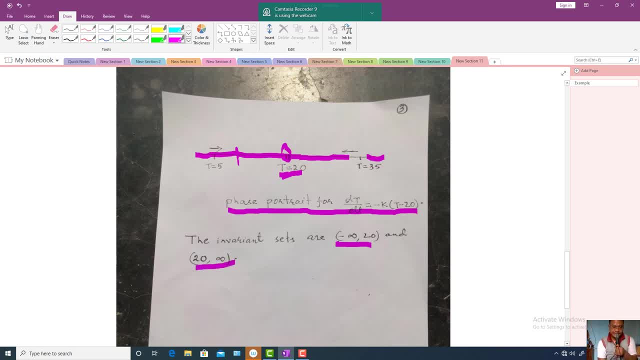 and this is also open set. so this is the fixed point. okay, this is the fixed point. in a way, fixed point can be regarded as a invariant set. okay, trivial fix, you know, trivial invariant set. so they are close, but generally invariant sets are, you know. you know non-trivial invariant sets are so 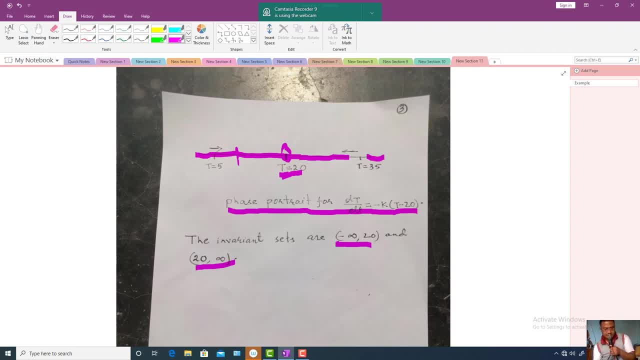 open set, open intervals, open sets, open intervals. right. so this is the concept of you know, if you know the invariant set, what does? the behavior of the thing is that if the if a set is invariant, okay, no point in the set will move out of the point, okay. 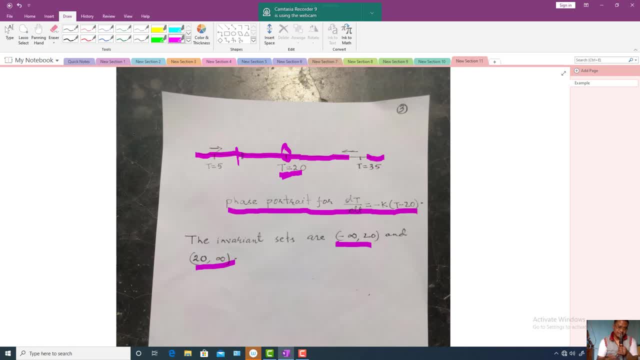 right, the behavior, you know the, the dynamics or the motion of the motion of any point inside the invariant set will be, you know, inside the set itself, that is, it is called invariant. okay, that is why it is very important first to find out the fixed point and then invariant set. all right, so 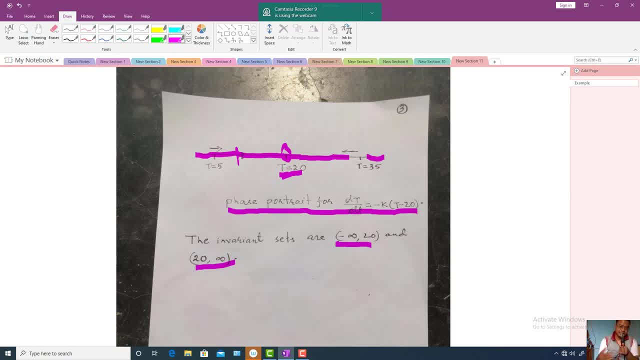 this, this is, uh, you know, this is the thing. now we have seen one real example, physical world example, and the appropriate mathematical, you know, equation is written and then we analyze, you know, we first find out the fixed point. we now, we want to know the solution of the fixed point, you know. so the name suggests that temperature. 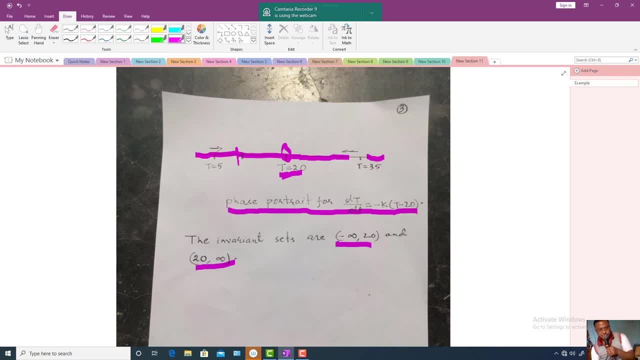 remains there and the solution also. you know, the solution also verified it. okay, so what is happening in the real world is verified by the mathematical equation. so this is the case of a good, good model, good mathematical model, or something like that. so this is, you know, this is about an